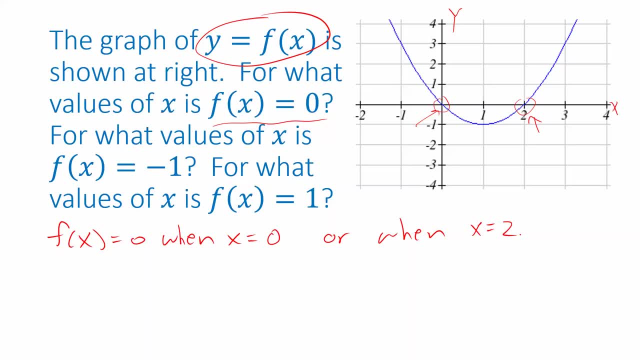 And now these might just be considered approximations because we're getting them from the graph. But for a question like this, you're typically supposed to assume that if the graph looks like it goes through a point that's easy to read, probably it's meant to actually go through that. 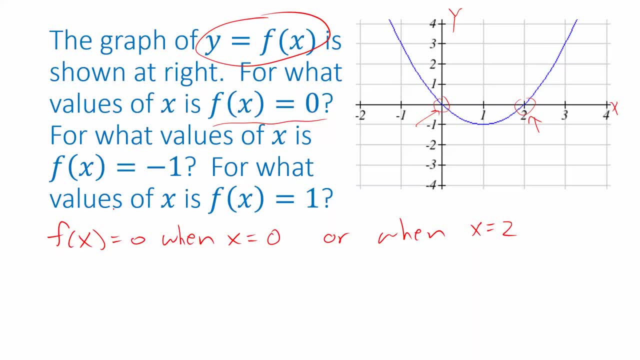 point. So let's take a look at a couple more. When is f of x equal to negative one? Well, we want to figure out. where does the graph line up with y equals negative one? Now, that's this line, and we see it appears there's one point on the blue graph that touches. 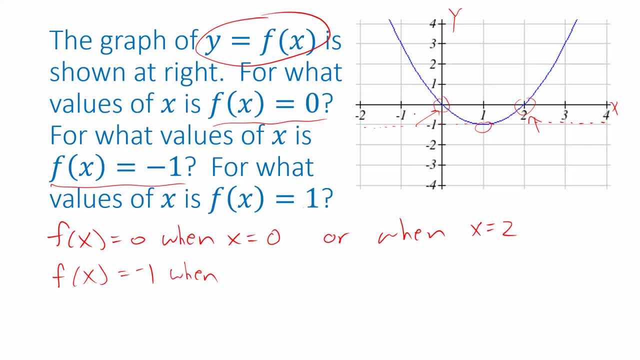 a height of y equals negative one, and that's when x is one. And then when is f of x equal to one? When is y equal to one? Well, that's up here at these two points, And now, when we look at these, it doesn't appear that it lines up with an exact value. 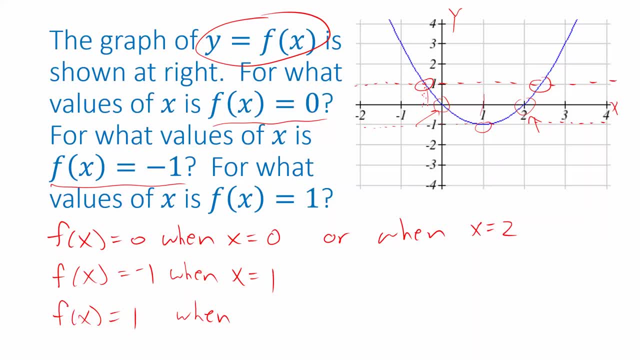 So we're going to have to estimate This x value. it's negative, it's less than zero. It doesn't look like we're quite at negative point five. We're a little bit to the right of that. So I'm going to estimate. 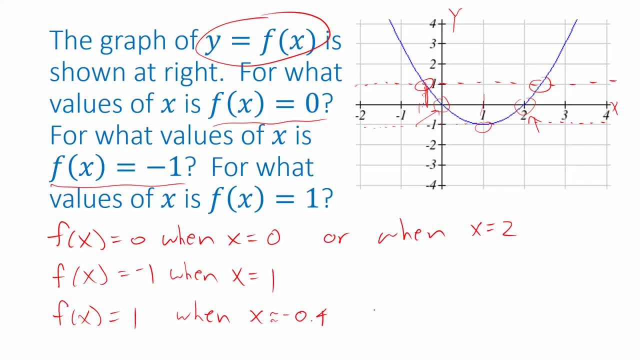 when x is about negative zero- point four. And the second point that looks to me like approximately two: point four. So a lot of times that's the best you can do: reading a graph. For more exact answers. you typically need to have a formula for the function so that you can solve an equation. 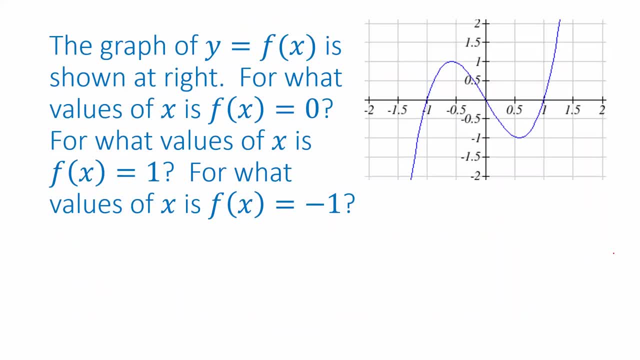 OK, Let's look at a few more examples. Here's another function: When is f of x equal to zero? Well, we want to know. when do we cross the line y equals zero, which is the x axis? That appears to be three points. 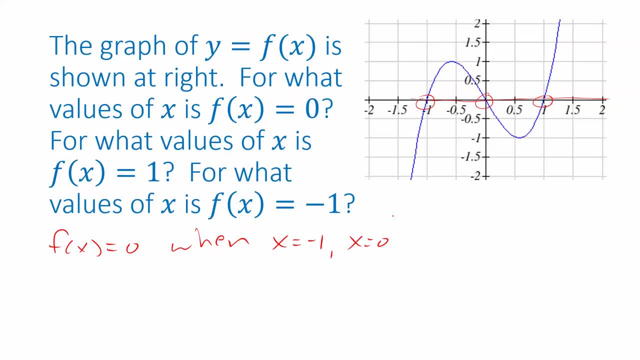 X equal to negative one, X equal to zero And x equal to one. Then when is f of x equal to one One? Again, We're going to have to estimate that It's at a point that's a little bit to the left. 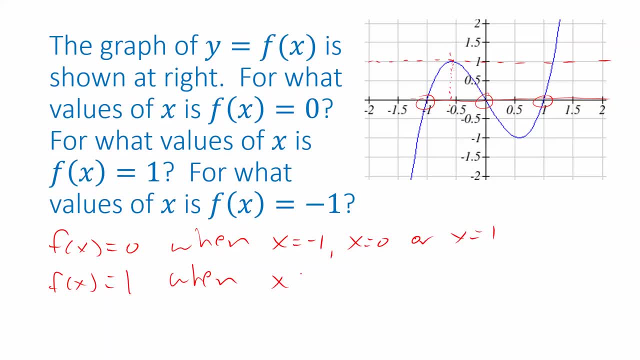 of negative point five On this scale, that looks to me like it's about negative zero point six. And when is f of x equal to negative one? Down here Again, that looks like it's a little bit more than zero point five On this scale. let's. 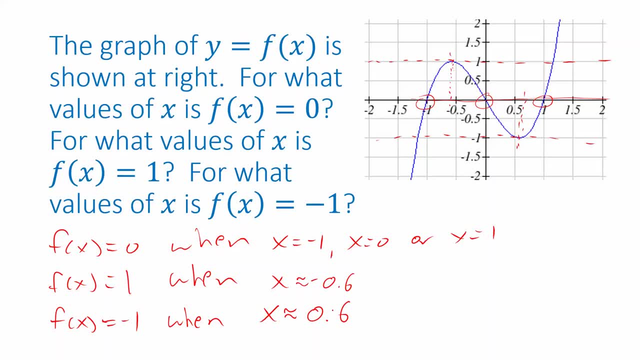 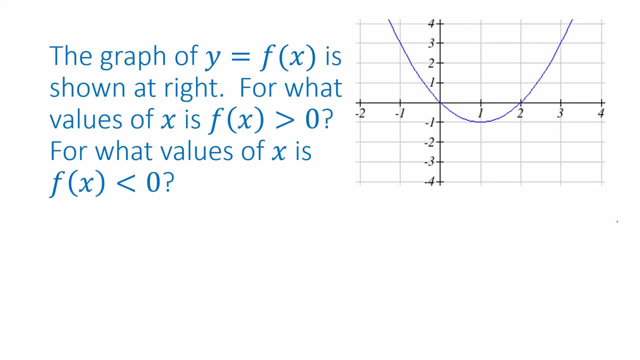 call that zero point five. OK, Zero point six. So this question is a little bit different. It's asking for what values of x is f of x positive? When is y positive? So we're not looking just for one value of y, We're looking for lots of values of y. 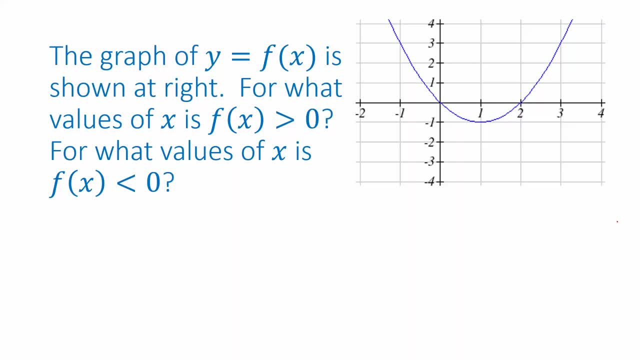 Everywhere where the function gives you an output that's greater than zero. That means that's everything here. So we want all of the outputs above the x axis, And it looks like we get that here. So we have x values that are to the left of this crossing. 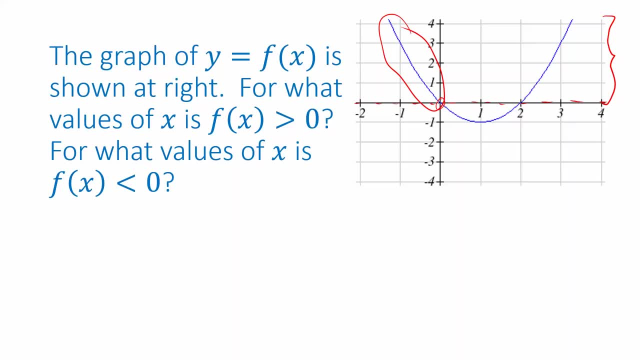 Now this crossing here, this crossing of the x axis, appears to occur at zero. We want what's to the left of that. So f of x is positive when x is less than zero. And we also want this part of the graph Which: 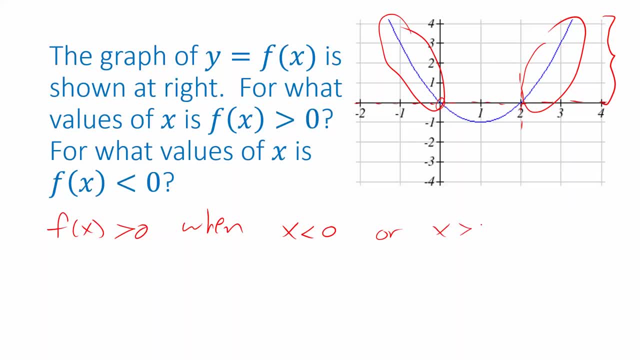 Occurs when x is greater than two, And then we're asked to figure out: when is f of x negative? That's going to be this region here between those two points. So x should be greater than zero and it should be less than two. 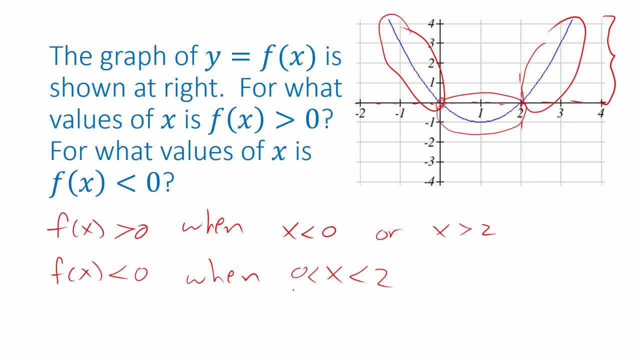 And you can express that and as just a single compound inequality like this: If I write These two inequalities- x between two values, This is the same as saying that x is less than zero and or x is greater than zero and x is less than two.